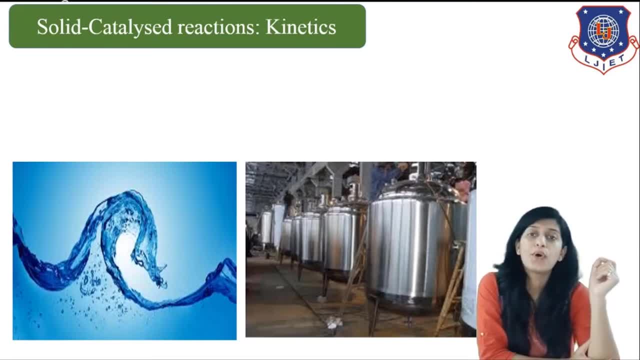 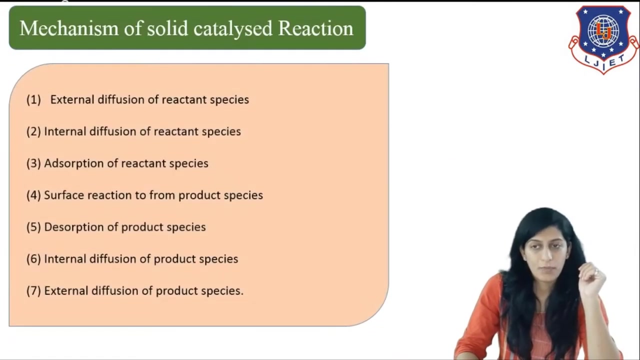 We are determining how to know which reaction step is the controlling step. So in this process only we have completed initial three steps and have seen how to determine rate of reaction for external diffusion, for internal diffusion and for adsorption. Now, in today's session, we will move forward and start our topic. 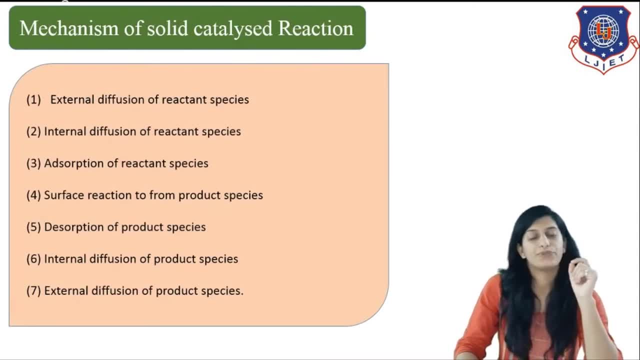 with step number four, which is surface reaction to form product. So, as we already discussed, we are having these seven types of steps which are essential to carry out solid catalyzed reaction. correct: Initially reactant has to diffuse from bulk phase to the surface of catalyst. 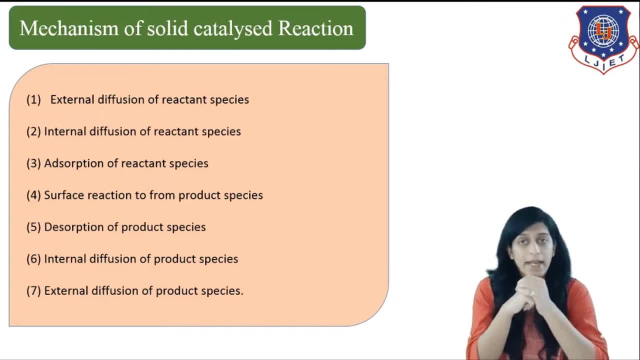 that is, to the external surface of catalyst right. Once the reactant has reached the external surface of our catalyst, then there will be an internal diffusion of reactant inside the pores of catalyst And this diffusion inside the pore when the reactant travel from onto the surface of catalyst to inside the pores of catalyst. 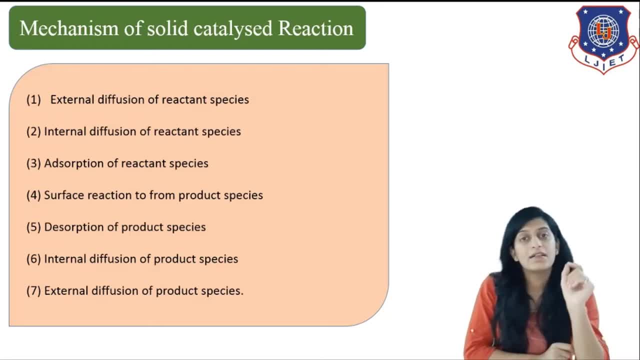 this journey we have termed as internal diffusion of reactant species, which is our step number two. right, They are diffusing from outer surface to inside surface of the pore. After that, there is step number three, which is adsorption of reactant species. 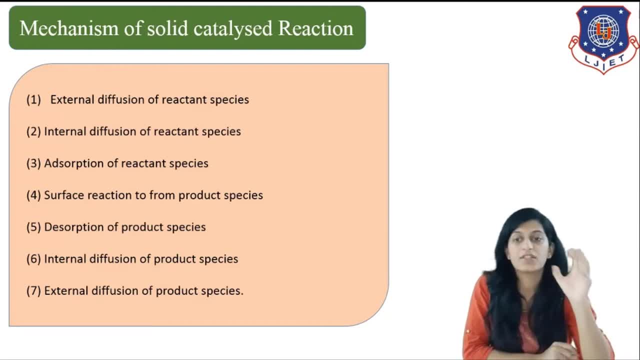 So in case of adsorption of reactant species, what happen is the reactant molecule which have gone inside the pores of catalyst. now they will try to get adsorbed on the walls of pore of catalyst, right? So they will now get adsorbed. 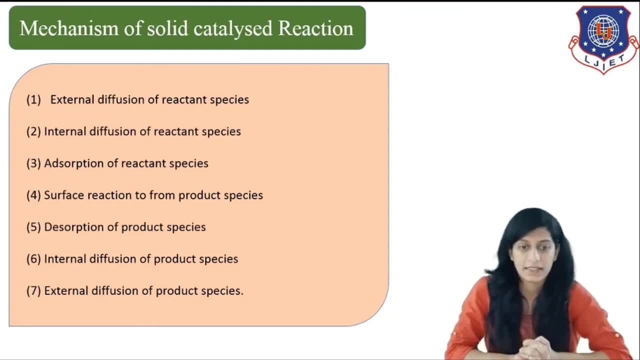 So they will now try to get adsorbed on the pores of catalyst, And this adsorption process of reactant is our step number three. After that there is step number four, which is surface reaction to form product species Once reactant are been adsorbed on the surface of catalyst. 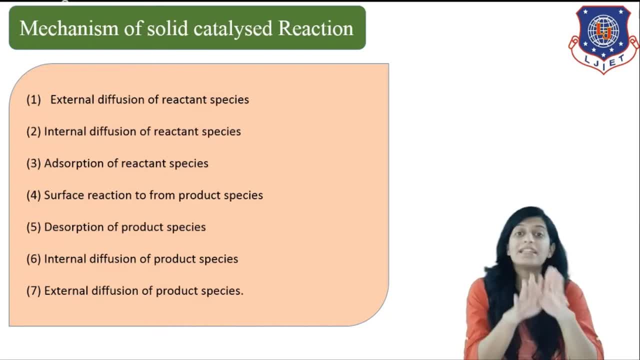 that is inside the pores of catalyst, then they are ready to react with each other and form desired product. Now this is our step number four. After that comes step number five, which is desorption of product species. right, Since reactant are adsorbed on the interior surface of our catalyst. 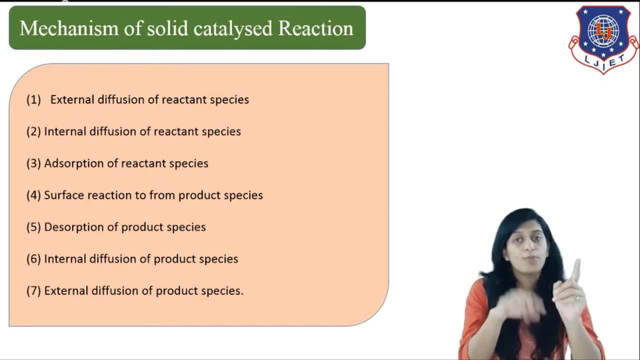 therefore, product will also be formed only on internal surface of our catalyst Right. So this is step number five, That is, product which is formed on the surface of catalyst, that is, inside the pores of catalyst, will now try to dissolve itself from the surface. 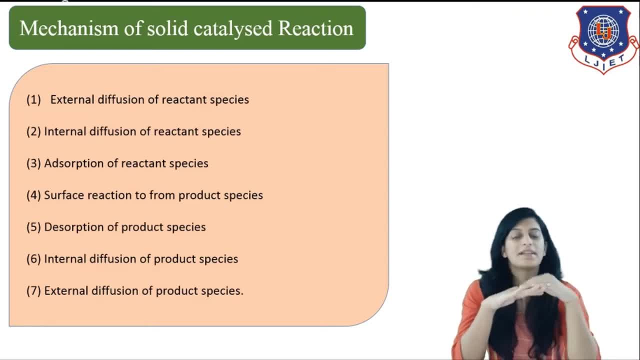 and come out of that particular surface. But this is happening inside the pore of catalyst, right? So this is step number five: Once product is dissolved from the surface or from the pore of catalyst, now it will try to come out of that particular pore. 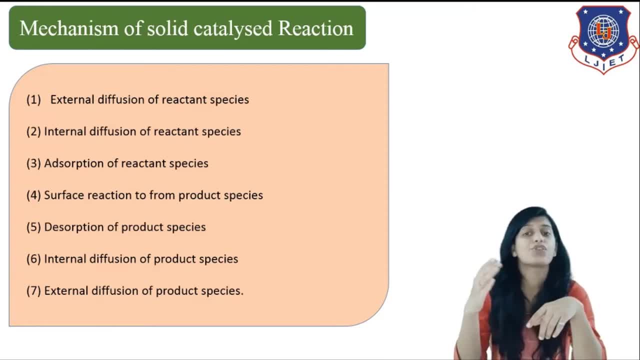 and this is known as internal diffusion of product species right. The formed product or the product which is formed inside the pore will now move from interior surface of the pore to the exterior surface of the pore and will come out of the pore. So this phenomena- 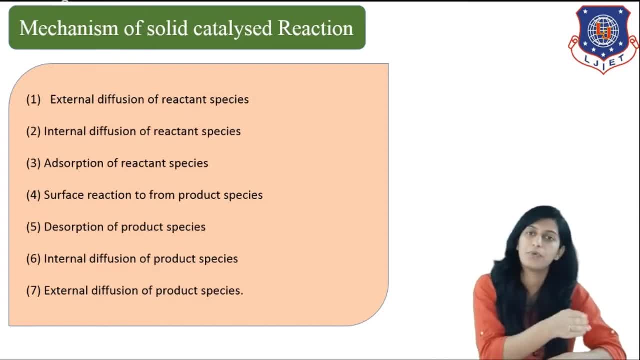 of travelling of formed product from inside the pore to outside the pore is termed as internal diffusion of product species. right After that, the last step comes, in which the formed product will now move from surface of the catalyst to the bulk phase, and this step is known as external diffusion of product species. 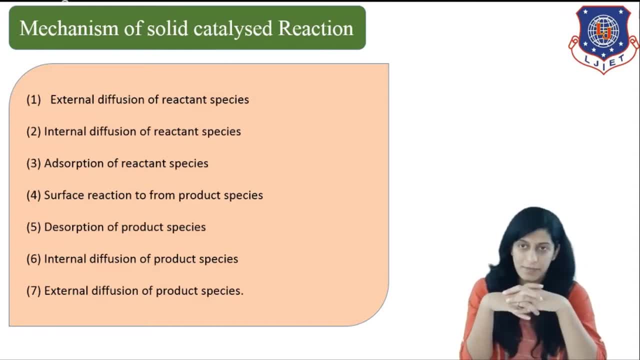 Correct. So these are seven steps. Now we need to determine, out of these seven steps, which step will control our reaction mechanism, right? So for that only, we need to understand the how to determine rate of reaction for given steps. So for step number one, step number two and step number three, 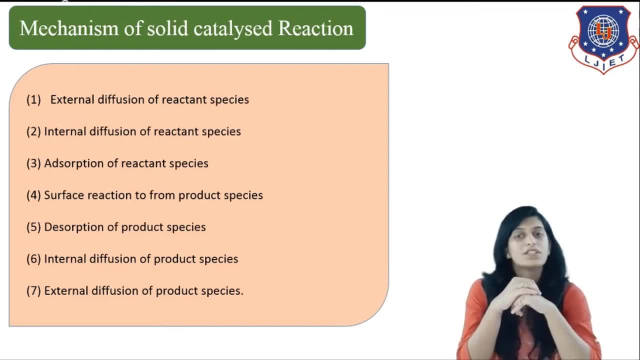 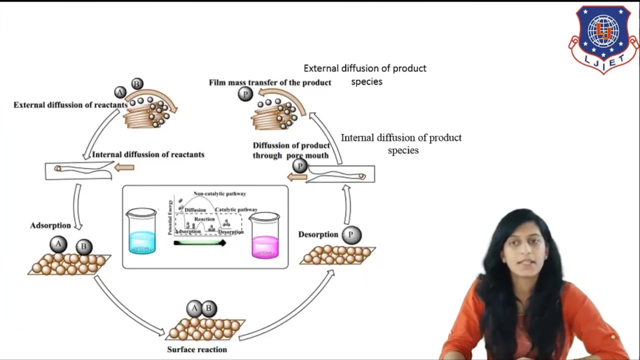 we have already seen the formula which is used to determine rate of reaction, and based on that calculation only we can determine the slowest step. Now in today's session we will start with step number four, that is, how to determine rate of reaction for surface reaction right. 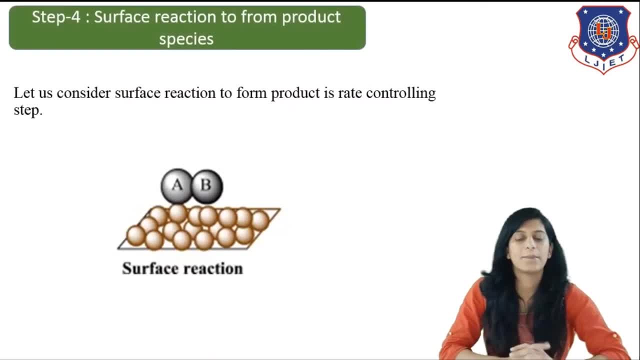 So now let us just start our step number four. So here we are considering that step number four, which is surface reaction to form product species. This is our slowest step. So as you can see in this particular picture, also that reactant A and reactant B, 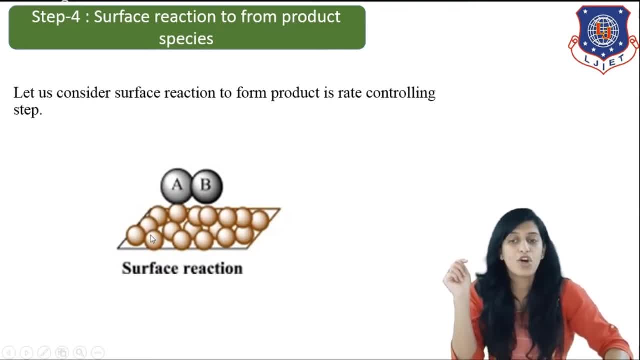 at this particular moment, both the reactant are adsorbed on the surface of catalyst- This brown shaded thing is catalyst surface- and A and B are the reactants. So A and B, both are now adsorbed on the surface of our catalyst, correct? 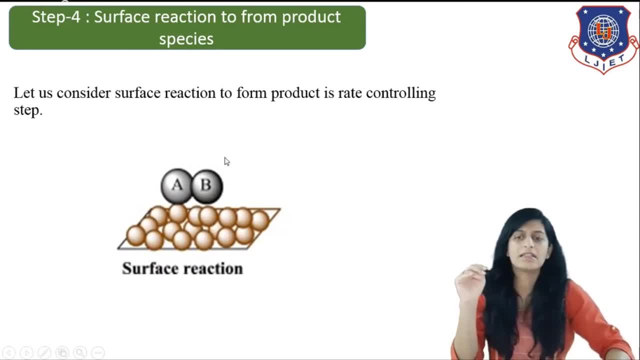 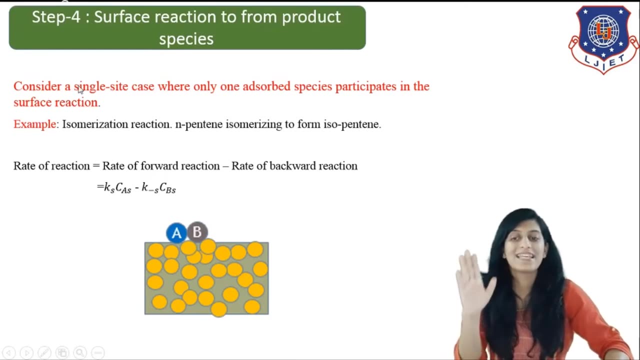 So now we are considering here that this is the slowest step. So what will happen if this is the slowest step? How to determine rate of this particular reaction? So for this we can consider single side case where only one adsorbed species. 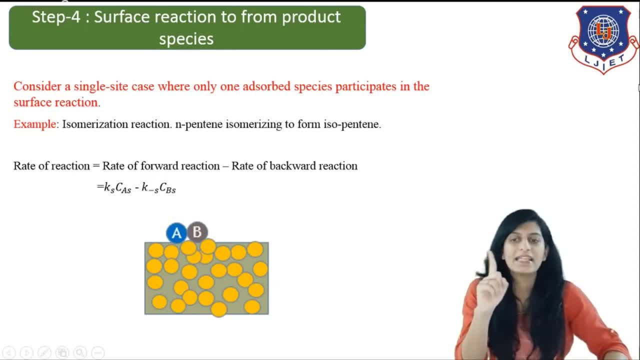 participate in surface reaction. We are saying that only one adsorbed species, that is A, is taking part in the reaction. So rate of forward reaction minus rate of backward reaction can be determined and that will be our rate of reaction right. So rate of forward reaction can be given as: 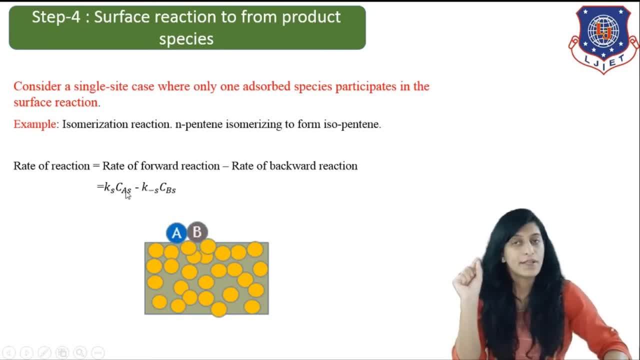 Ks, that is rate constant into concentration of component A in the solid phase. that is Cas minus K minus S, that is rate of backward reaction into concentration of B in the solid phase. That is why it is written as CBS right. So this is the case when we are considering. 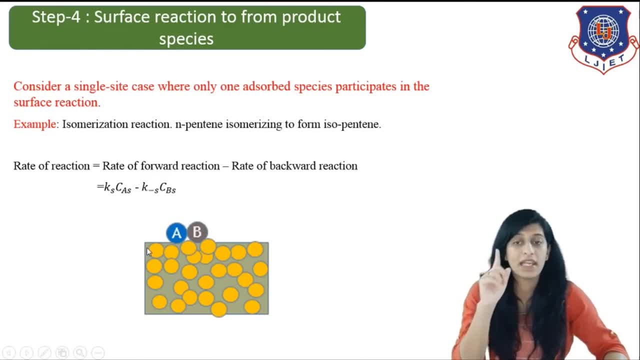 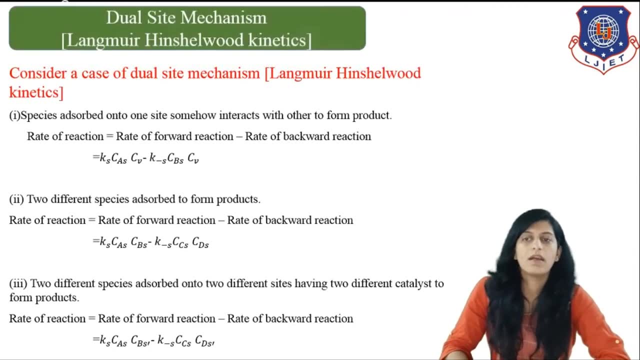 single side case, that is, in the single side only Reactant are adsorbed and getting converted into product. Now the next topic, which is quite essential and very important, is dual side mechanism, or it is also known as Langmuir-Risenwald kinetics right. 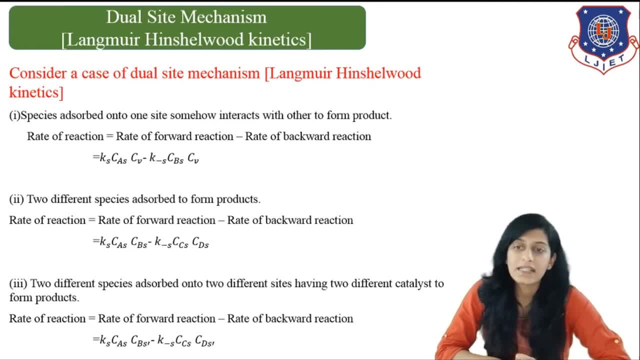 So for this here we are considering that there are two different sides which are being occupied and involved in formation of product. right Before this we have seen only single side is combined and utilized for formation of product, But in this particular case we are considering that two different sides. 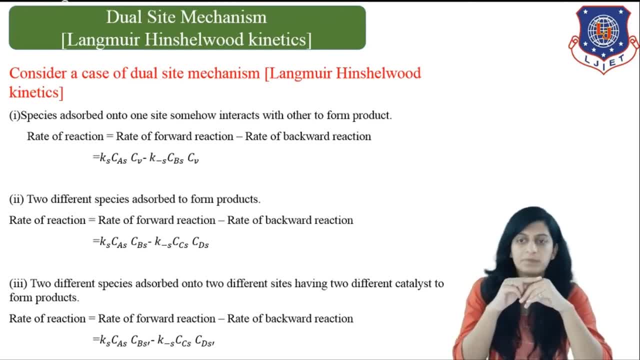 are involved in formation of product. So, as you can see here, first case is species adsorbed. Species adsorbed onto one side. somehow it will get interact and it will form the product. So this is case number one: Species will adsorb on one side. 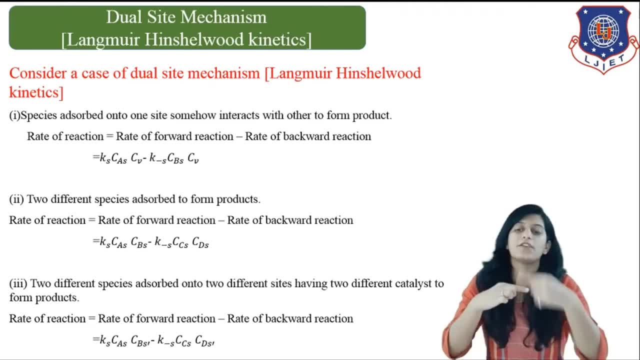 and then they will come in contact with each other and form the product right. Next case will be when there will be two different species and they are getting adsorbed to form product. In this particular case, it is considered that in this single pore 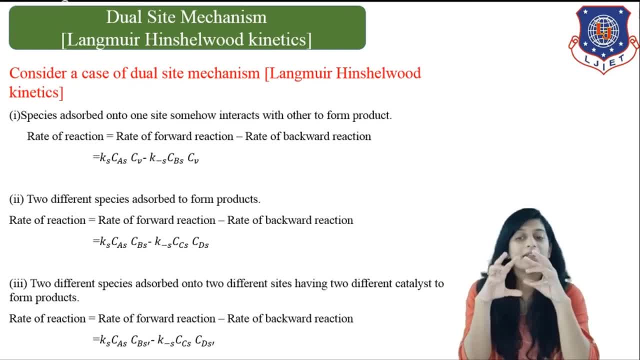 both the species are getting adsorbed and they will form intermediate and that intermediate will then jump into the another pore and then it will be forming the final product. So this is case number two, when two different species get adsorbed to form product right.